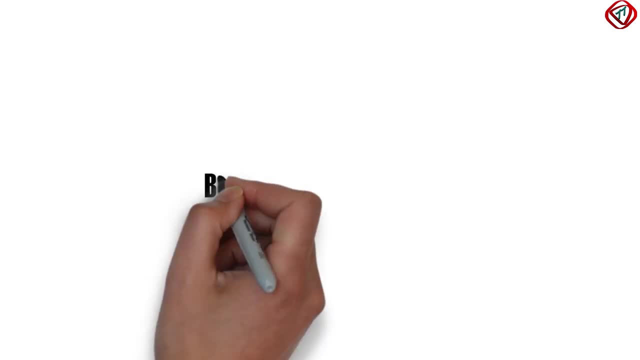 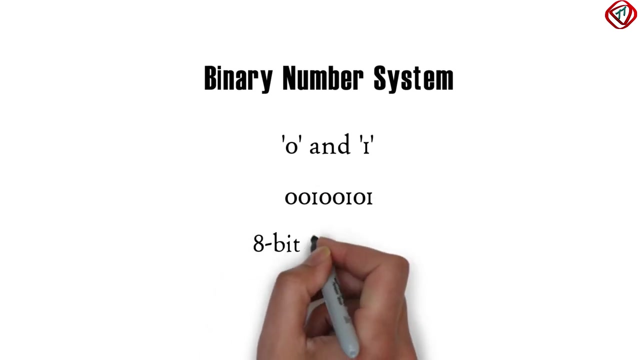 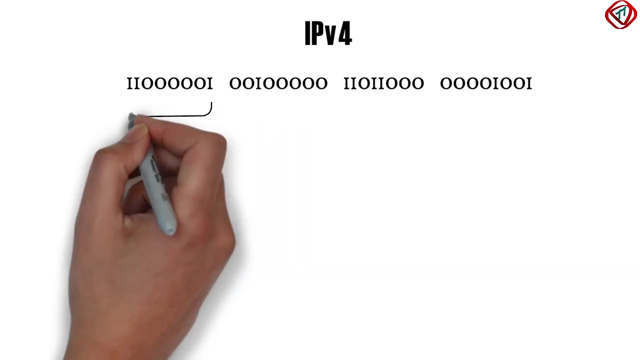 and not with host and router. We know that this binary number system uses two symbols: 0 and 1.. If write a sequence of zeros and ones, for example 00100101, say, it is 8 bit in length. Similarly, IPv4 address is 32 bit in length. 8 bit represents 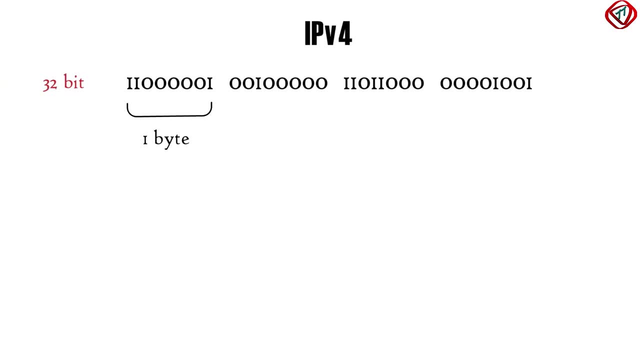 1 byte. Therefore, IPv4 is 32 bit or 4 bytes in length. Each byte is written in the form of decimal numbers separated with dots. This notation of IPv4 address is called dotted decimal notation. Now, a portion of this IP address is determined by the subnet to. 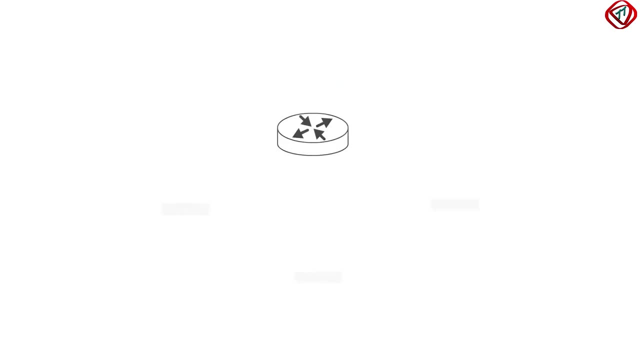 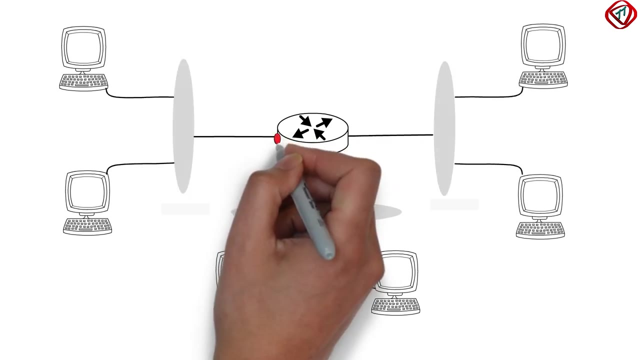 which the device is connected. Consider: a router is connected to 6 hosts via Ethernet switch or wireless access point. The router has 3 interfaces and each host has 1 interface. Each interface has its IP address. Please note that each host interface and the router. 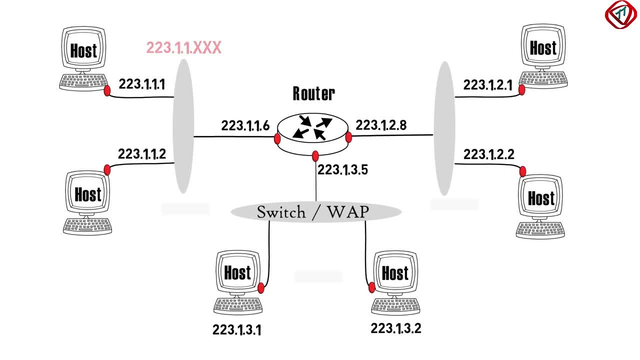 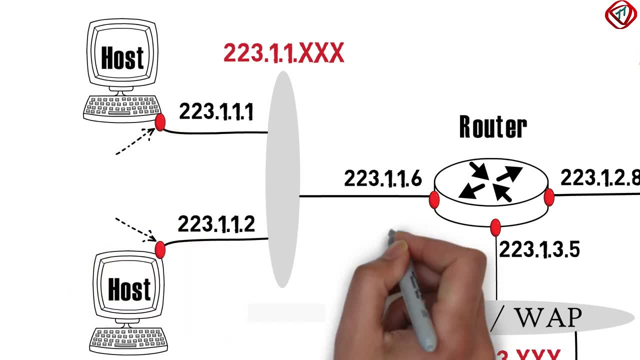 interface to which hosts are connected has the same IP address format. The network connecting the host interfaces and one router interface having the same IP address format is called subnet, and here it is represented as 223.1.1.0.24, where slash 24 is known as subnet mask It. 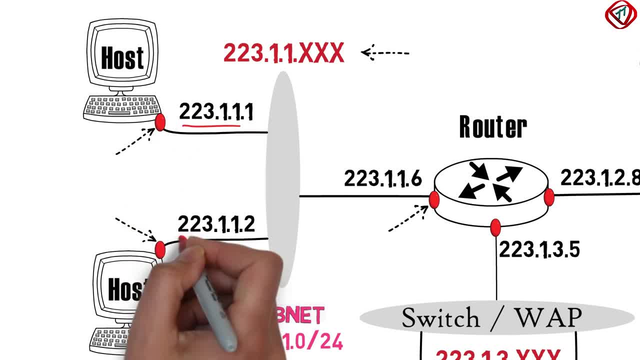 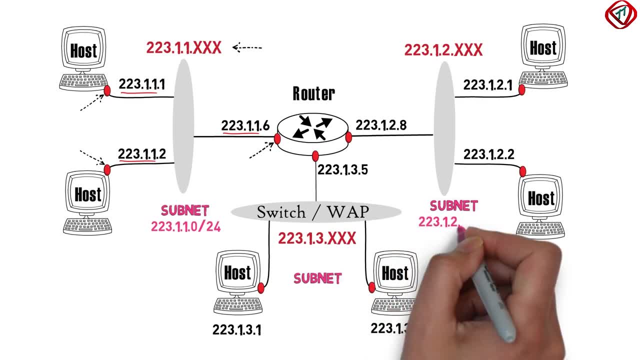 means that all interfaces in the subnet have the same IP address format. This means that all subnets have the same IP address format. Similarly, two other subnets are 223.1.2.0- slash 24 and 223.1.3.0 slash 24.. An organization has multiple subnets where each subnet has 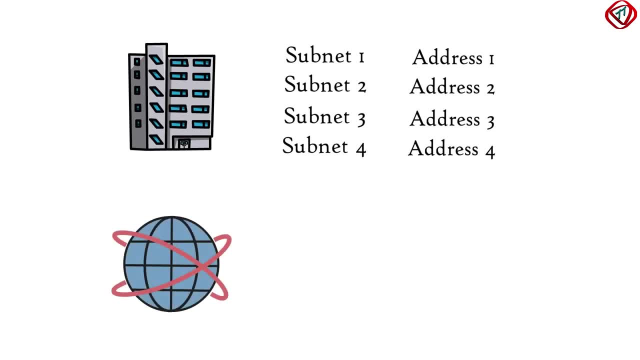 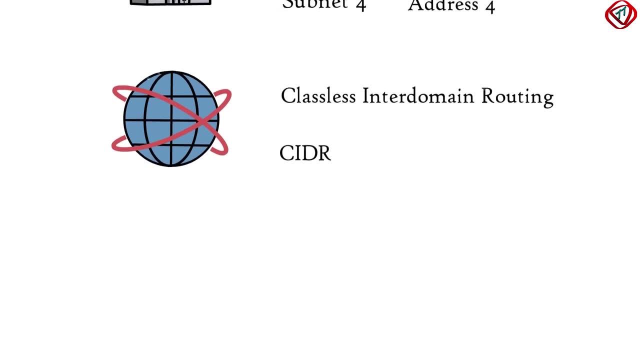 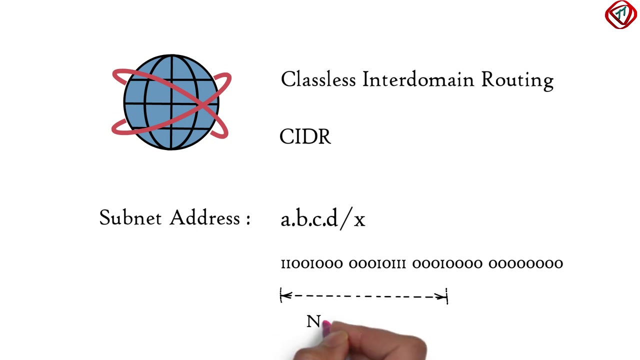 a different address. In the global internet the IP addressing is handled by Classless Inter-Domain Routing or CIDR Address Assignment Strategy. In CIDR, addressing the subnet address is generalized to abcdd, slash x, where x indicates the number of bits from left, The first x bits is called network prefix: An organization.